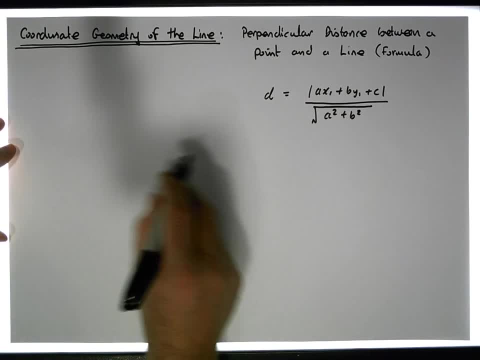 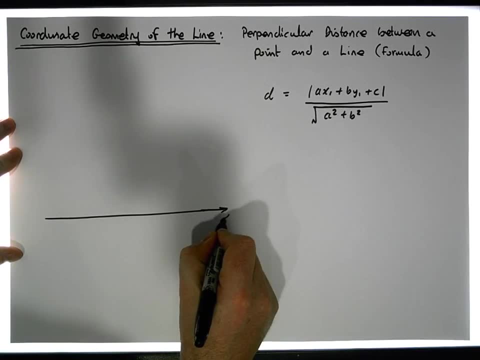 Let's just geometrically, let's just have a look at this Graphically. yeah to a coordinate system. Okay, so let's say we have an x-axis here. let me just extend it out. We have an x-axis and we have a y-axis which is perpendicular to the x-axis. okay, 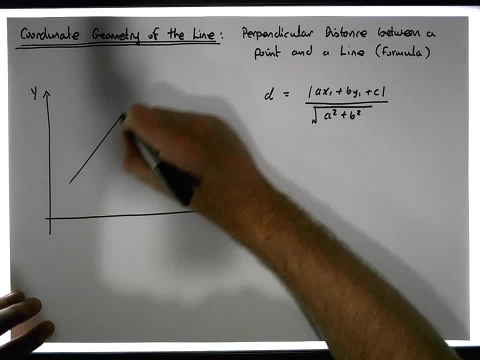 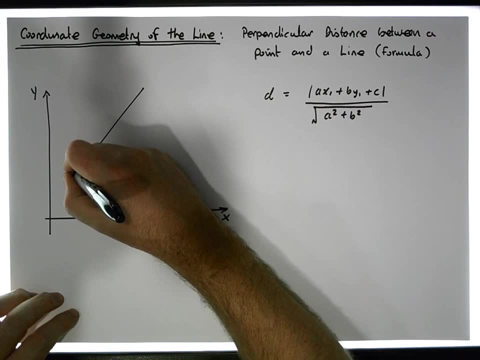 And let's say we have a line in space. let's just say we have a line here, something like this: Let's call this line, let's say just there's a line, okay, and let's say it has an equation of a line. 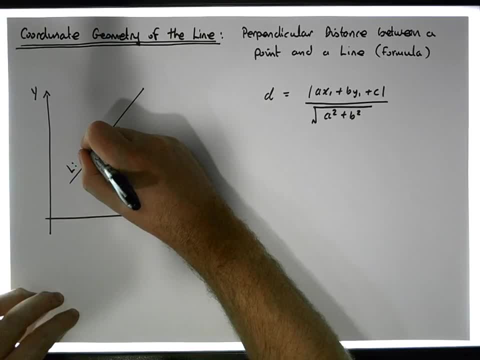 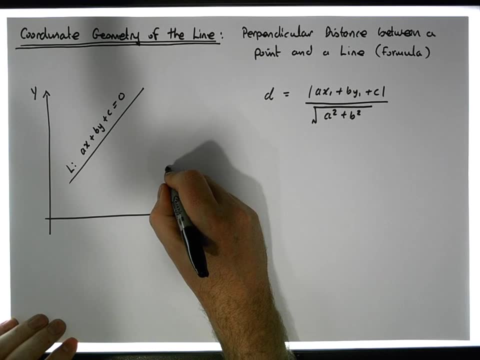 Let's call it L, okay. and let's say the equation of the line is ax plus by. Let's say it's equal to zero. okay. And let's say we have a point in space. and let's say the point in space is somewhere. let's say here, okay. 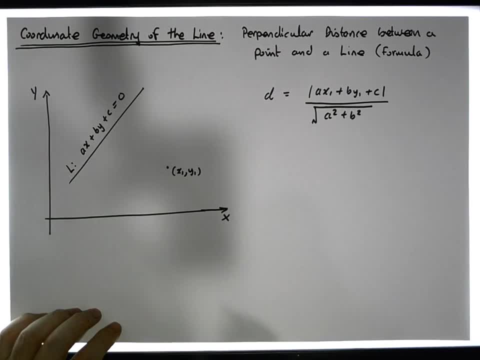 And let's say, this point is x1, y1, okay, And what we're interested in is we're interested in how far this point is away from this particular line, But, more importantly, what we're interested in is we're interested in the perpendicular distance, okay. 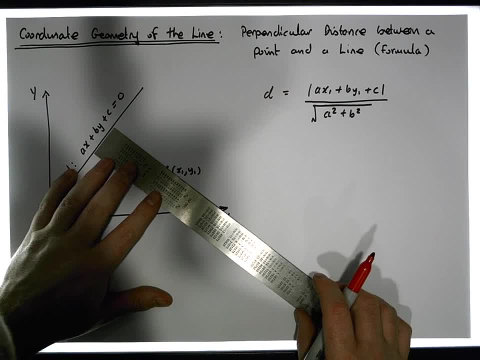 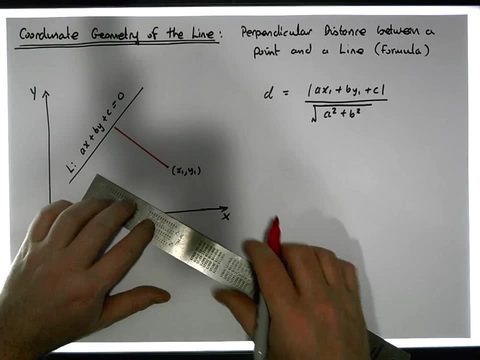 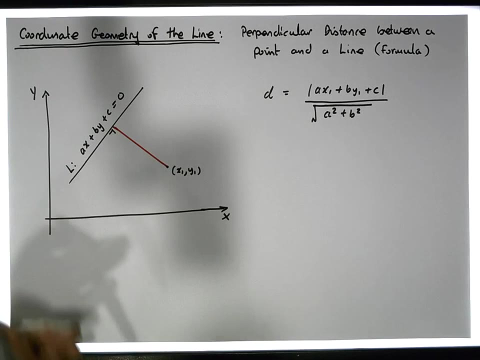 So we're interested in the perpendicular distance for the line, the point and the line. So we're interested really, and what is this distance here? if that makes sense, what is that distance here between that point and this line? and this is a perpendicular distance. okay, now we do know how to calculate distances. 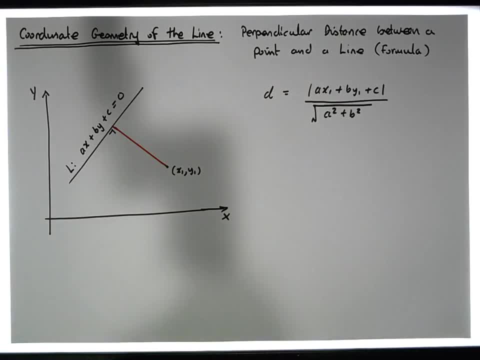 and we know how to calculate distances when we have two points and we calculate the distance between two points. okay, so the first thing maybe that we should do is we should try to find another point, because we have a point x1, y1, and maybe what we should try to do is to try to find the point. 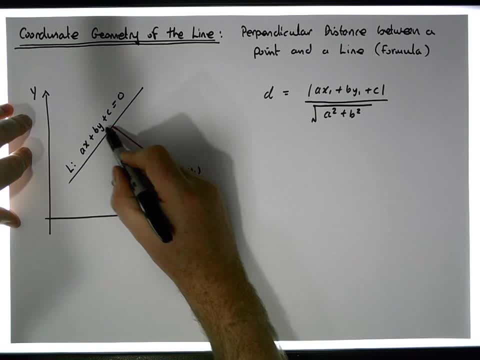 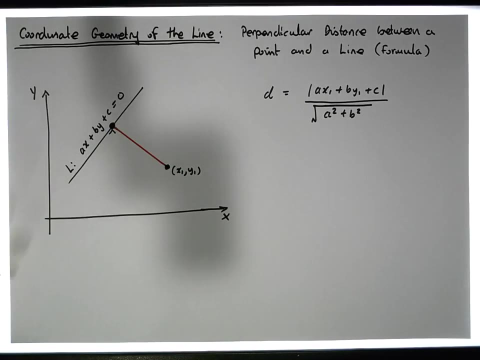 along this line that intersects with this, with this particular, this particular line here, this line segment, where this line segment is perpendicular to this line l? okay, so we know this particular point here: x1, y1. why don't we try to find this particular point, this particular point here and 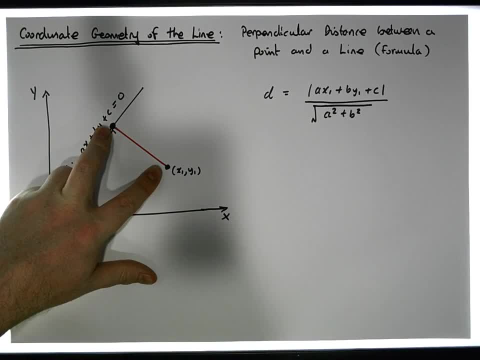 once we have them, two points. we can use the distance formula to calculate the distance between the two points, which is the perpendicular distance that this point is away from this particular line, this particular line l, and we can use the distance formula to calculate the distance between the two points, which is: 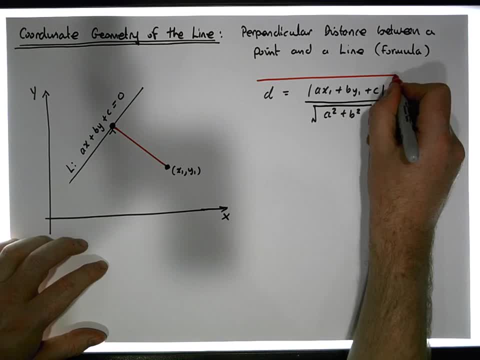 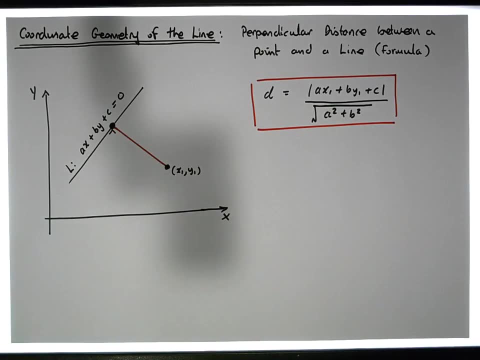 What I'm saying here is that it's actually given. it's given by this particular formula here, okay, And what we'd like to do is we'd like to derive this particular formula. There's a lot of work in this, a lot of algebraic work, okay, first of all, 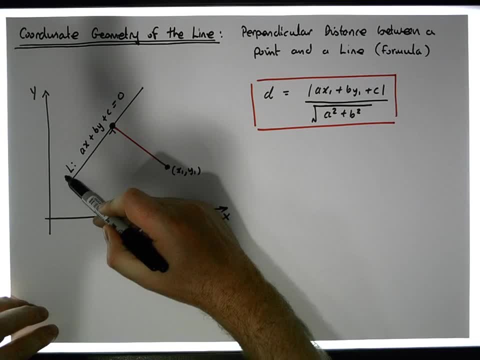 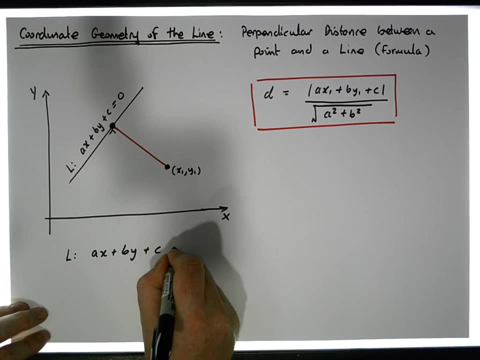 Okay. so let's say: well, we know that this line here is the line L, it's AX. The line L is AX plus BY plus C equals 0, that's the line L. It's just a general line. it could be anywhere in space, okay. 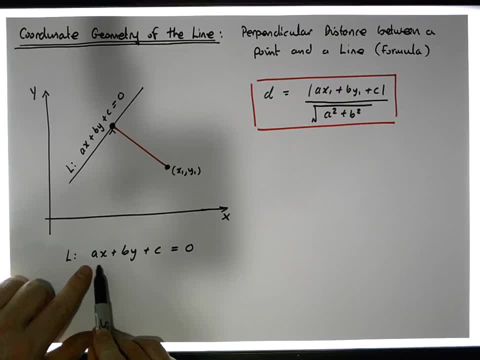 But it has a particular slope, and in particular the slope of this line here is minus A over B, so it's minus A over the B. A line perpendicular to it- let's say M, a line perpendicular to it, will have an equation that looks like this: 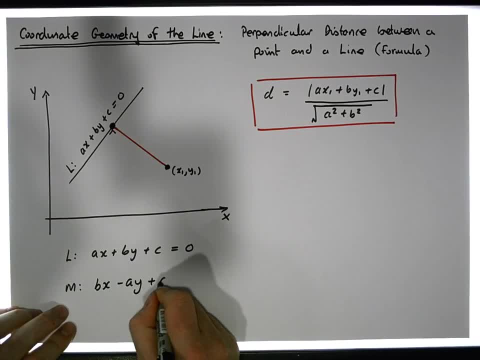 It's BX minus A, AY plus some other constant D, it must be equal to 0.. These two lines are perpendicular to each other. okay, Simply because the slope of this line here is minus A over B and the slope of this line here 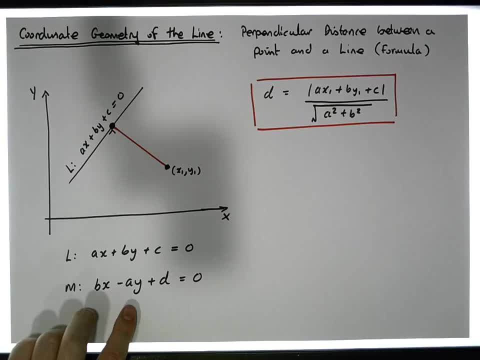 It is minus B over minus A. okay, which is B over A, if that makes sense? yeah, okay. So when we multiply them together, we actually end up with minus 1, which shows that this line is actually perpendicular. You can check that out yourself. 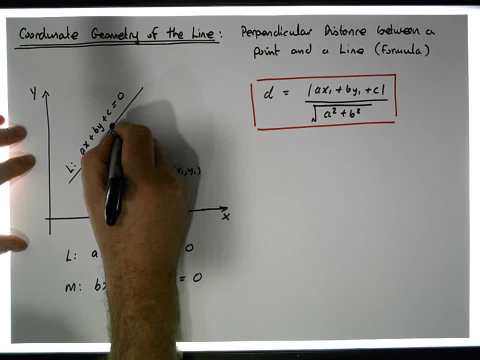 But the main thing here is this is: let's call this particular perpendicular M and let's say it's defined by this equation, which is: BX minus AY plus some number, D equals 0,. okay, So we have some general equation. we don't know where it is. 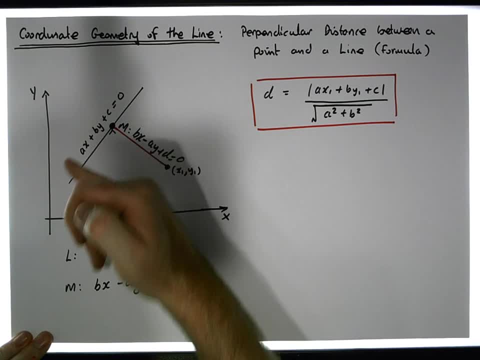 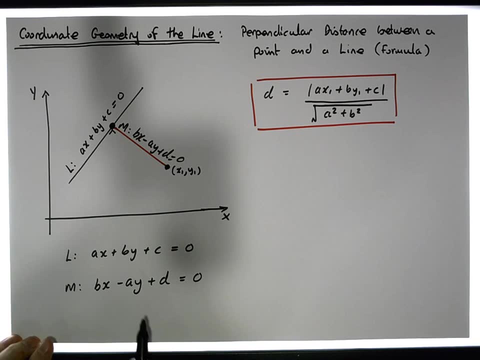 This is a general equation, so it could be anywhere along here This line. okay, but what we do know is that this particular point- X1, Y1, is on the line. So because X1, Y1 is on the line, that means that X1, Y1 must be a solution, okay. 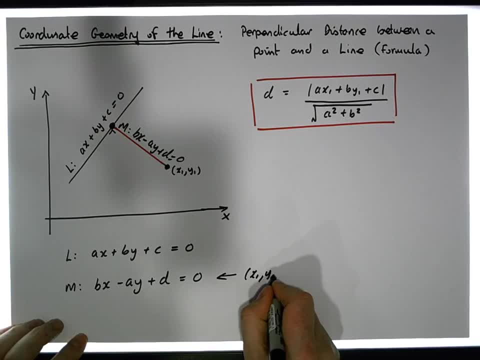 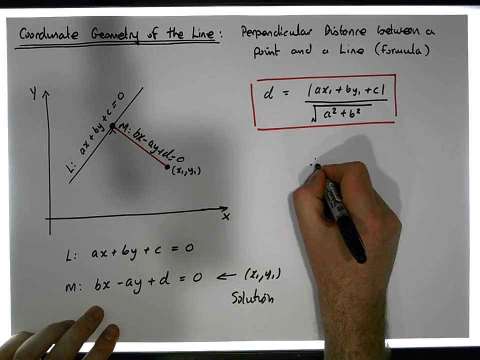 So X1, Y1 must be a solution, okay, to this particular equation. okay, So what does that tell us? Well then, therefore, okay, we must have that. if it's a solution, it means, when I substitute in X1, Y1, I should get 0.. 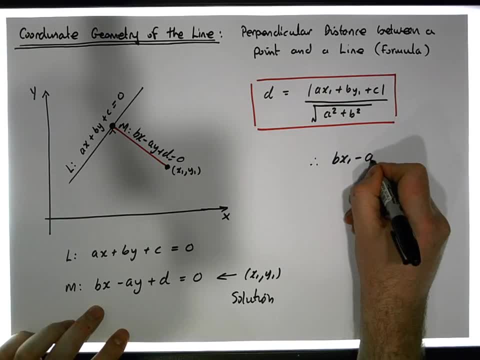 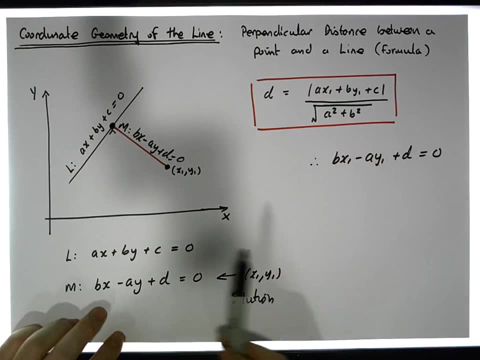 So that means that BX X1 minus AY1 plus D must be equal to 0,. okay, Now we can solve for D. we don't forget: we'll be given, you're going to be given when it comes to these problems. 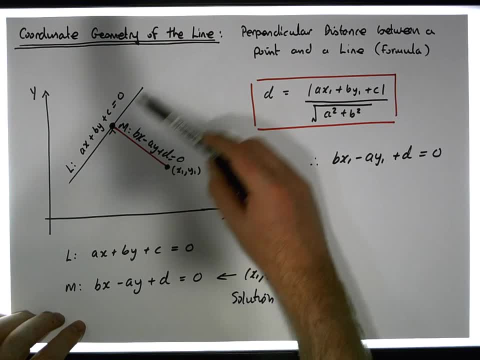 you'll be given a line AX plus BY, plus C, and you'll be given a point X1, Y1.. So, for all intents and purposes, we know A, we know B, we know C and we know X1 and we know Y1.. 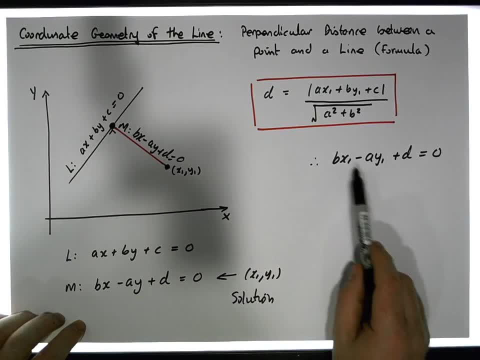 So out of this particular equation here, the only thing that we actually don't know is D, so we just solve for D. Now that D must be equal to, well, let's keep the positive term first. so it must be equal to AY1 minus BX1. 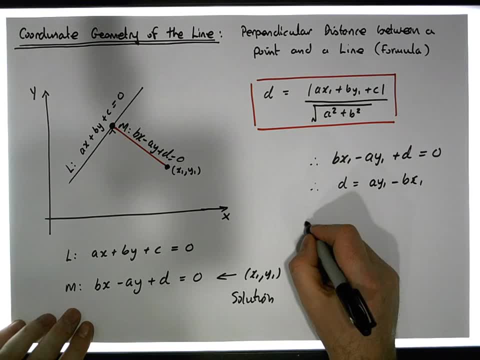 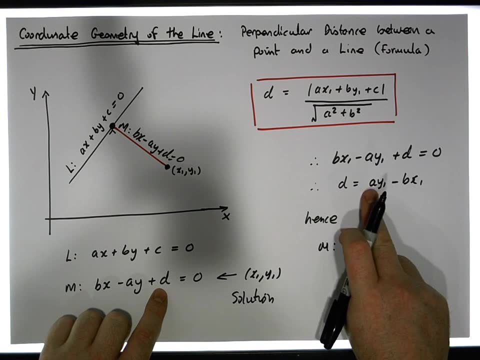 That's what D must be equal to, And hence and hence, hence, M must be this particular equation now, where we now know the D value in terms of the A's, the B's and the X1's and the Y1's. 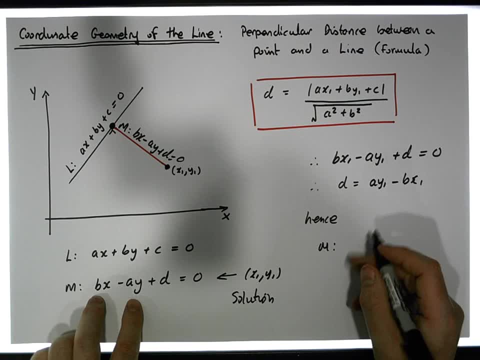 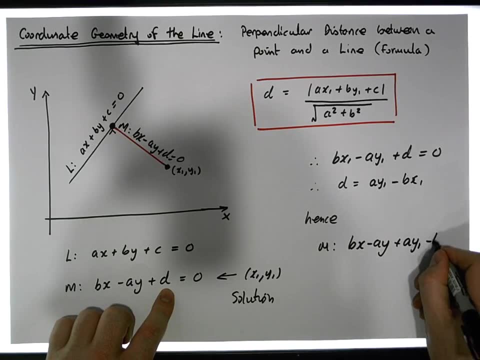 So now we know that M, the equation of the line M, must be BX minus AY plus D. well, D is plus AY1, minus AY1, minus BX1- must be equal to, must be equal to 0.. 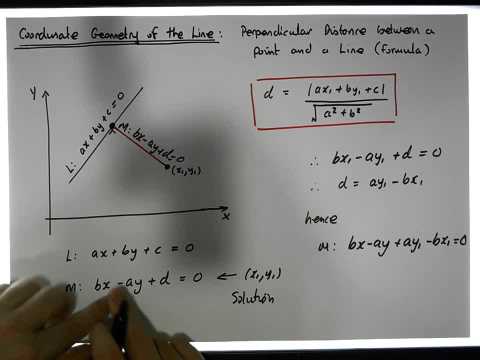 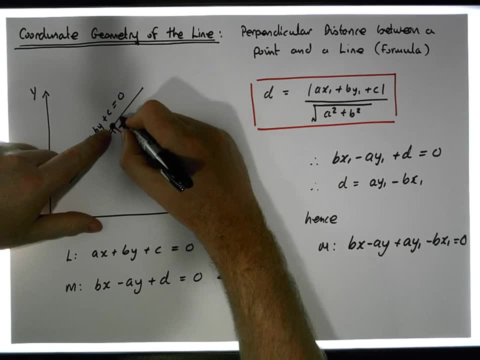 Okay, So, for all intents and purposes, now we have two equations of the lines. We have the line L and we have the line M. so why don't we find our point of intersection which will give us, which will give us this point here? 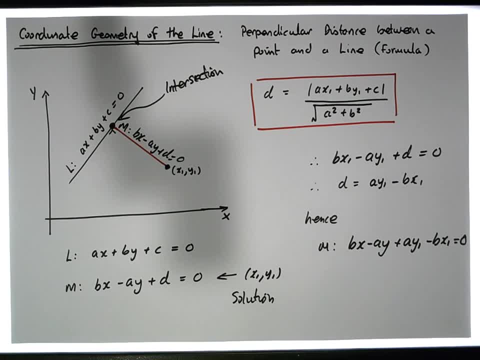 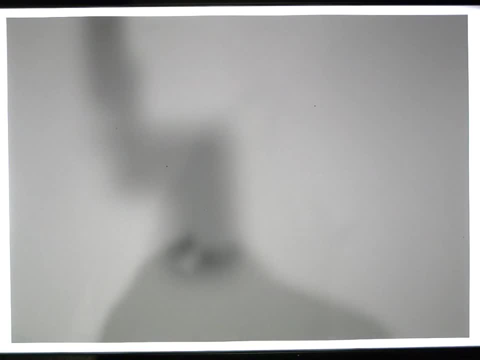 the point of intersection of these two particular lines. Now, this is where things get a little bit crazy from an algebraic perspective, but things should be okay. Okay, Things should be straightforward enough. So let me just write down these two lines again. 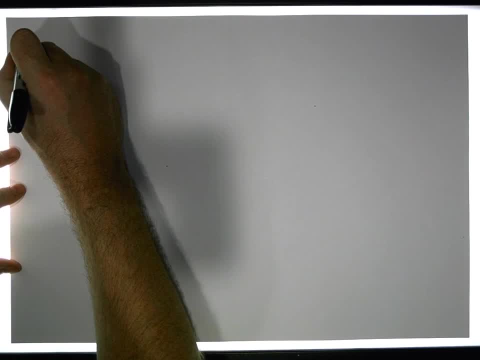 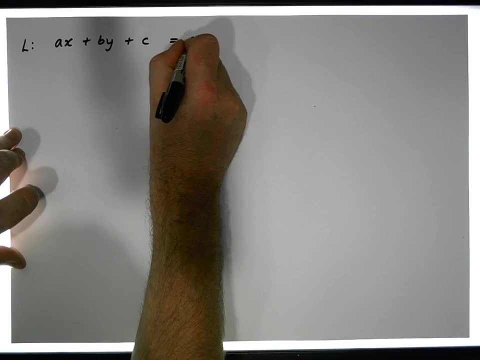 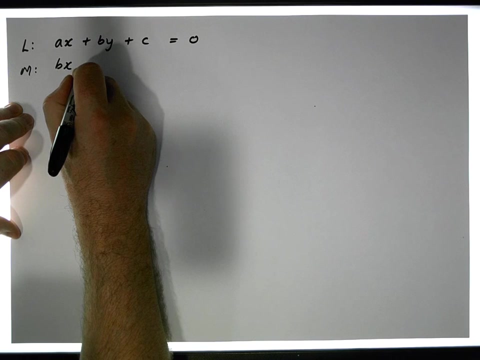 Okay, let me just write them again. So we have L- L. the line L is: it's AX plus BY plus C equals 0.. And the line M: the line M is BX is BX minus AY minus AY. 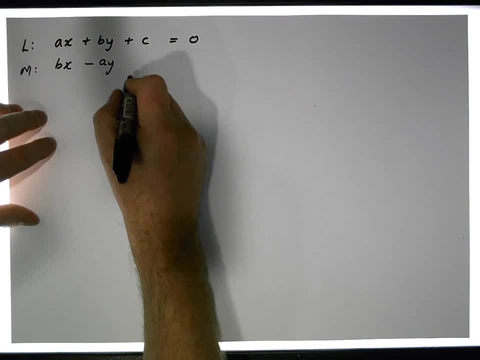 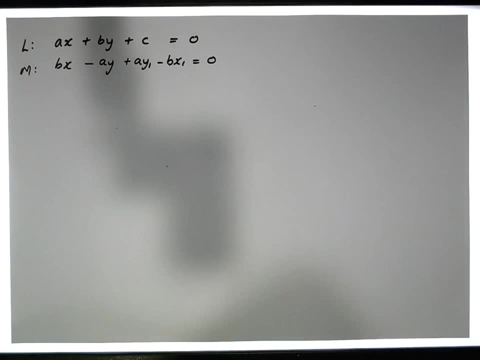 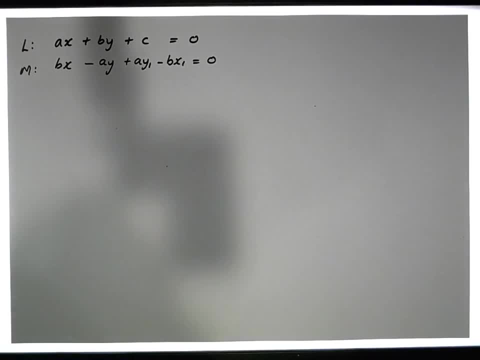 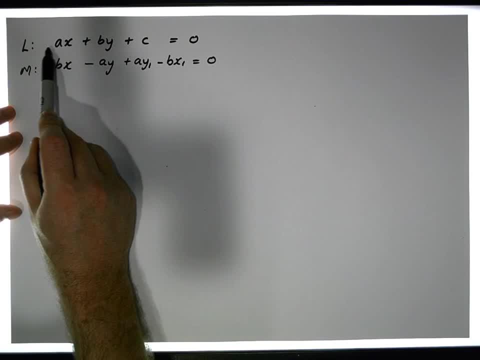 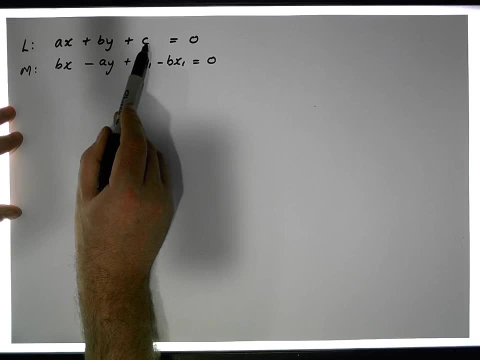 Let's get rid of the X's first and solve for Y. So let's divide L by A, That will make this, in the form of X plus some factor of Y plus some other term, is equal to 0.. And let's divide M across by B.